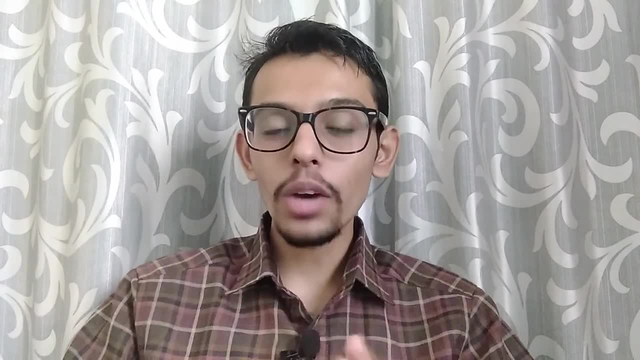 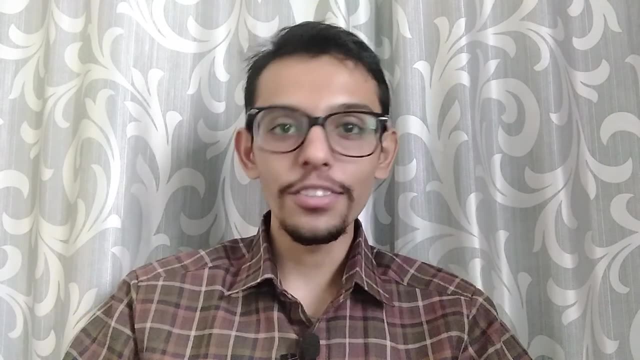 on the upper. i button or down in the description box. Neural networks are the building block of deep learning, and convolutional neural networks are built on top of it. So it is important to understand that concept first, And I think you should also subscribe to my channel, because I 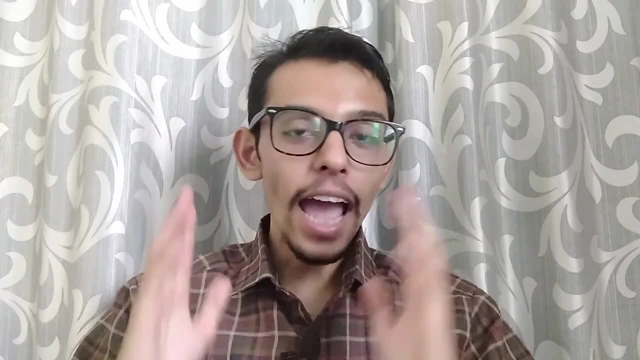 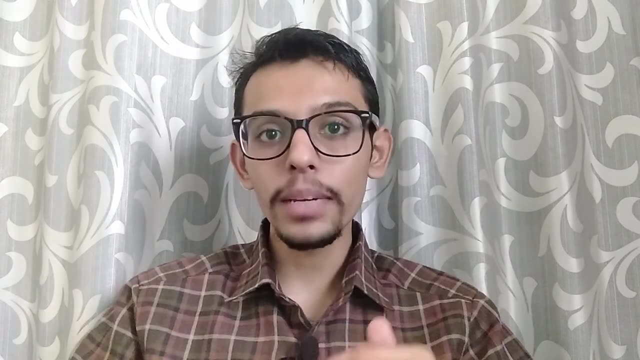 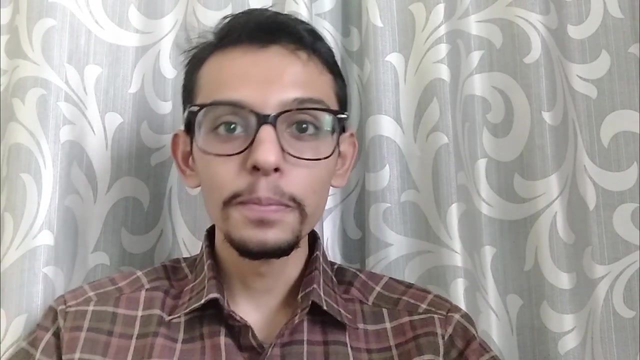 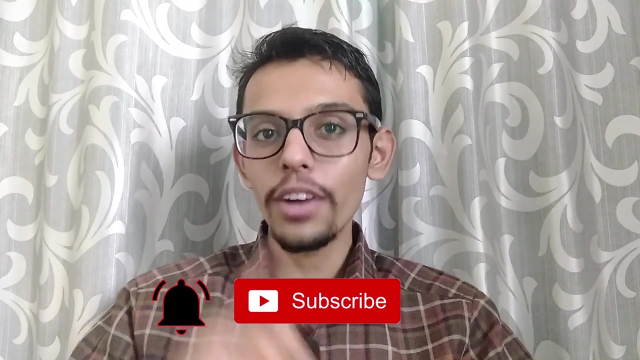 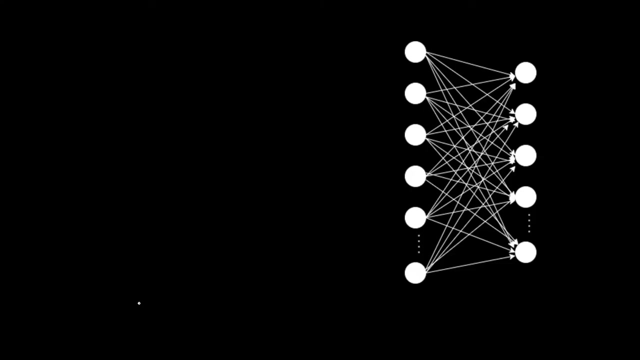 appreciate your support. Thank you for watching this video and I will see you in the next one. Let us see what is the drawback of using a simple neural network and why do we need a convolutional neural network in the first place. Let us say we are dealing with the image data set. 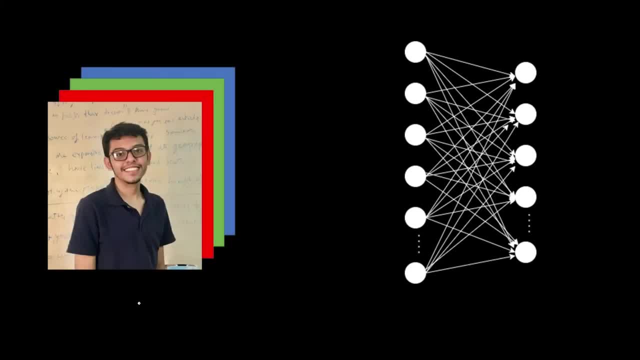 and it has colored images with red, green and blue channels, RGB channels having the size of 1000 cross 1000 pixels. Thus the total number of input features in this neural network will be 3 into 1000, into 1000, which will be equal to 3 million input features. And let's say, the first hidden layer in 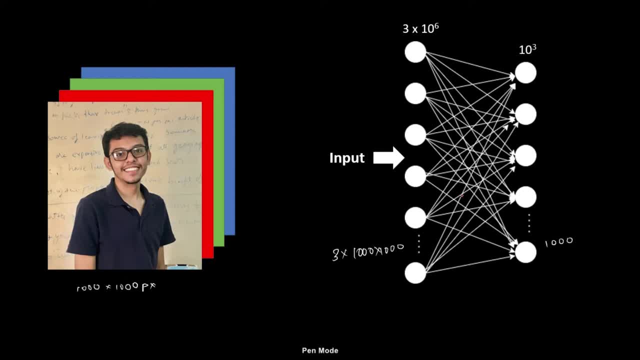 our neural network has only 1000 number of features, Then the total number of connections, or the weight parameters between these two layers will be this multiplied by this, which will be 3 billion weight parameters- And these are a lot of parameters to train- and thus the number of 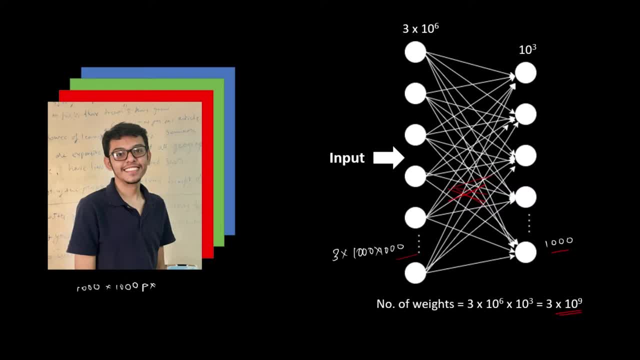 operations performed will be too large and our CPU or GPU might not be able to handle it properly. And even if it can handle properly, then also the time required to train the model will be very high. And by the way, more number of neurons and more number of weight parameters also means 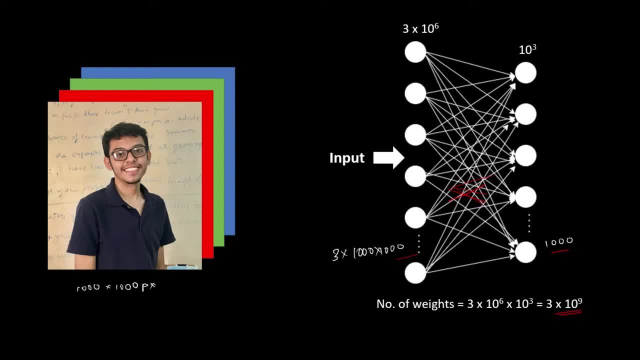 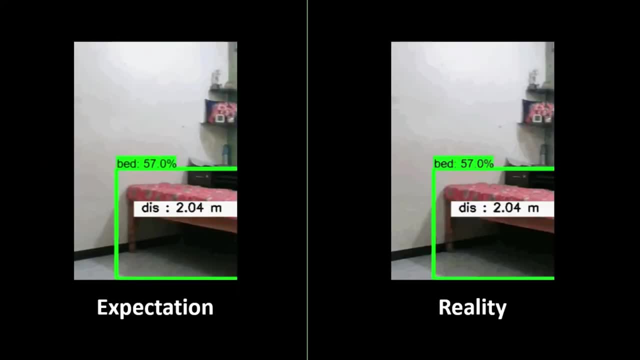 overfitting. Thus it can also affect the performance of our model as well. So this is the limitation of the traditional simple neural network while dealing with the images. Now just imagine if you were to perform some computer vision application like object recognition, then with such a slow speed of our neural network it will never be able to give a smooth expected. 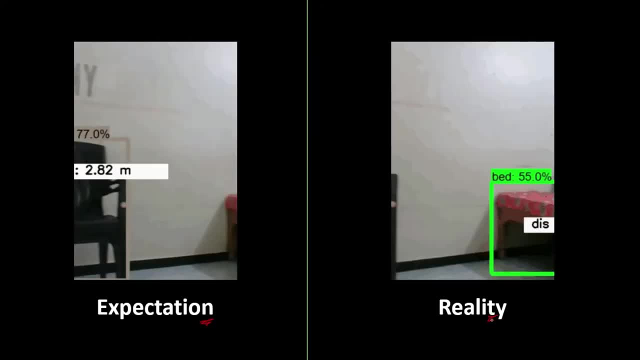 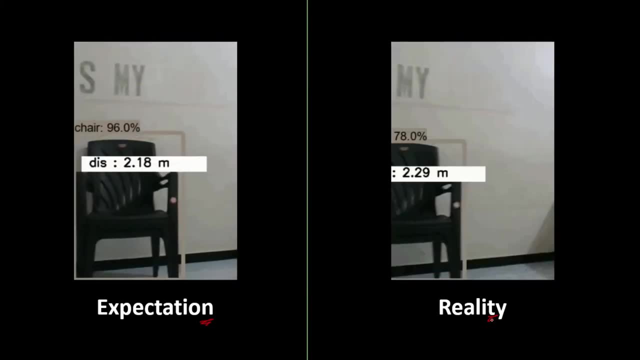 outcome, but it will keep lagging. So how do we do this? How do we overcome this limitation? Should we altogether not use the neural network on images? No, To overcome this limitation, deep learning community and researchers came up with this amazing concept called convolutional neural networks. 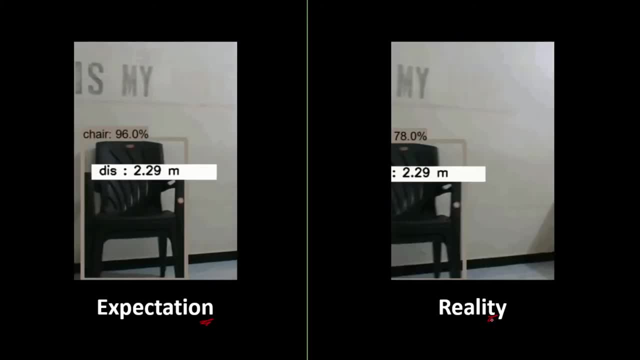 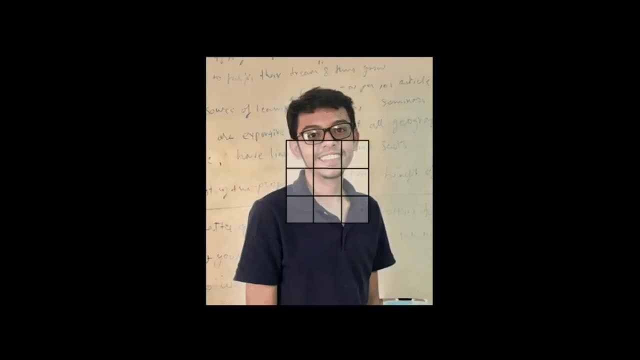 It is still a neural network, but it is a special type of neural network. The main idea behind a convolutional neural networks is using filters. Now these filters are sliding windows in our images that are responsible for detecting the features or patterns in the image. 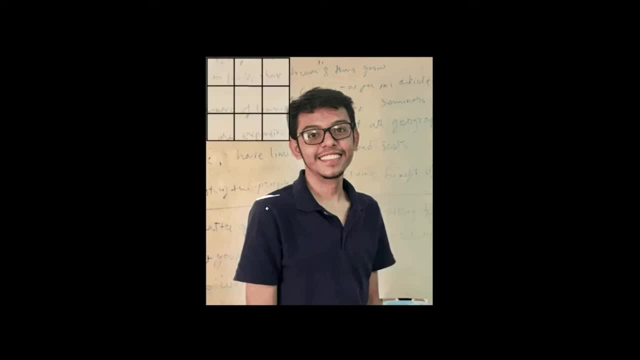 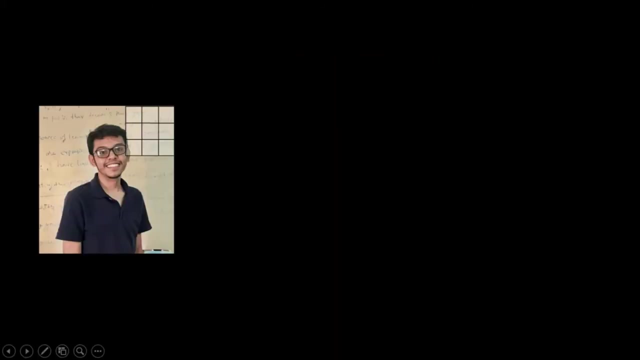 Now, image has this property that it has edges, it has shape, it has color and, with the combination of all these, it has features. These filters of the CNN will be responsible for detecting these features associated with the image. For example, this is a beautiful picture of mine, and when I 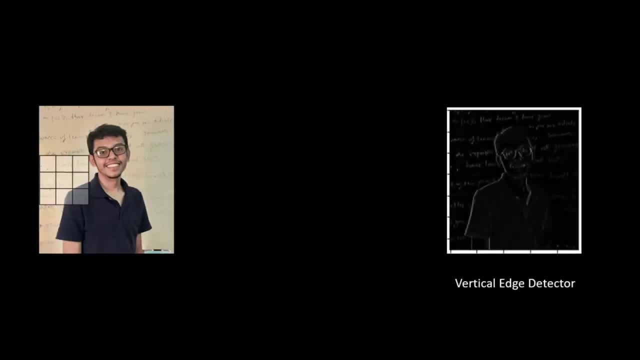 pass a vertical edge detection filter on this image, it generates me this image. It detects all the edges that are present in this entire image And similarly, if I slide over a horizontal edge detector filter of convolutional neural network, then it will detect me all the horizontal edges. 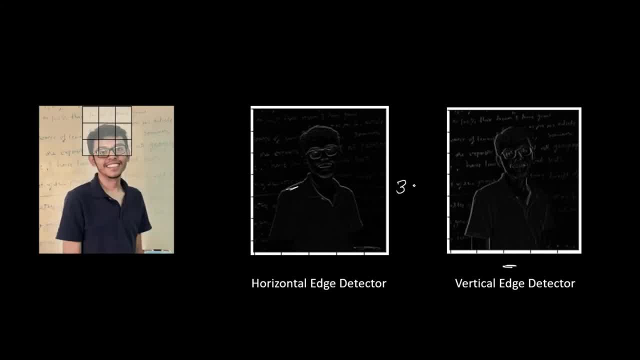 Now these two images are generated by using a filter of only size 3 x 3 pixels, So the total number of parameter in this are only 9.. Thus we are greatly reducing the number of parameters to train Now in a single layer of a convolutional neural network. we will be using lot of such filters. 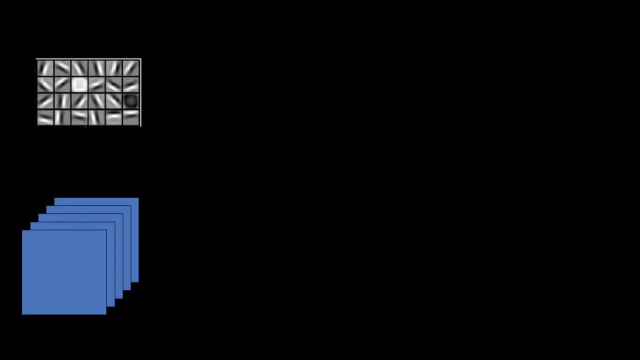 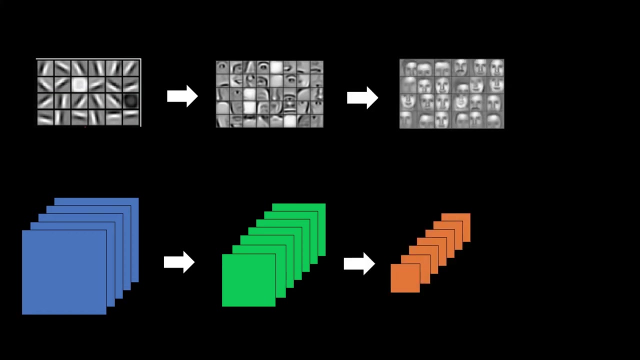 We will be using these filters to detect the edges all around our images. Now these edges will be passed on to the further layers, which might detect the features associated with the image, like eyes, ears, nose, etc. And, in the later layers, might detect the entire face in the image. by combining 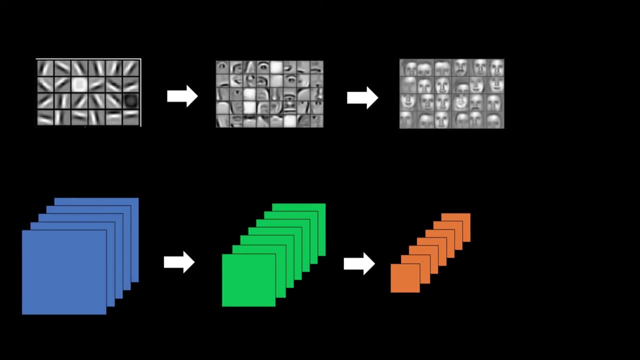 all the eyes, nose and ears. And once we identify these features, we can associate them to a particular label. For example, the feature of the face can be associated with the label human, And thus the next model sees a face in an image, it will automatically detect the presence of a human in it. So we are 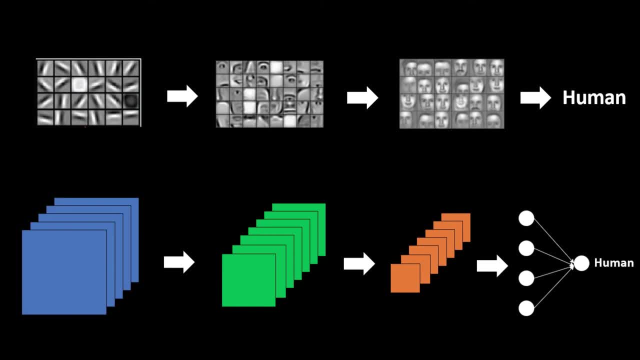 doing an extremely well job of identifying the features from the images, and the cost for this is just a few number of parameters. Thus, we have greatly reduced the number of parameters from 3 billion to just a very few. The only additional time it takes is in the sliding window, but it is. 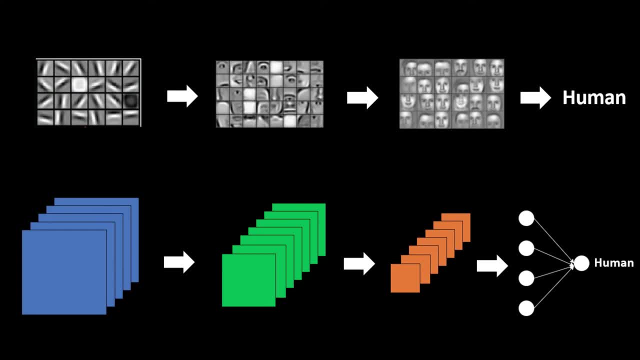 still much less than what it would have taken by using or training a simple neural network. So the convolutional neural networks are very powerful models while dealing with the images or videos and they perform exceptionally well than the simple neural network. And this is just an introduction to the convolutional neural network.